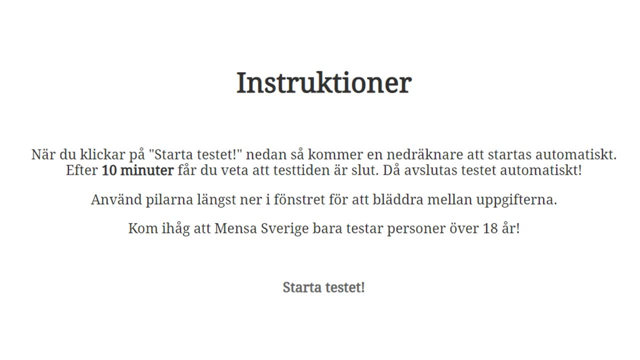 limit of 10 minutes, which is way smaller compared to the other Scandinavian Mensa IQ tests. For a comparison on how little time this test gives, the Mensa Sweden IQ test gives 25 seconds per puzzle, while the Mensa Denmark IQ test gives 62 seconds per puzzle, so above twice the time. 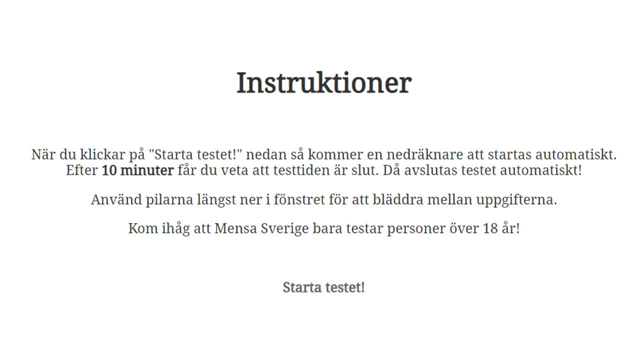 per puzzle on the Danish one. Overall, I found the test quite enjoyable. If you want to take the test yourself, the link will be in the description and if you're just following along, I suggest you pause the video before listening to my solution and try to solve it yourself. 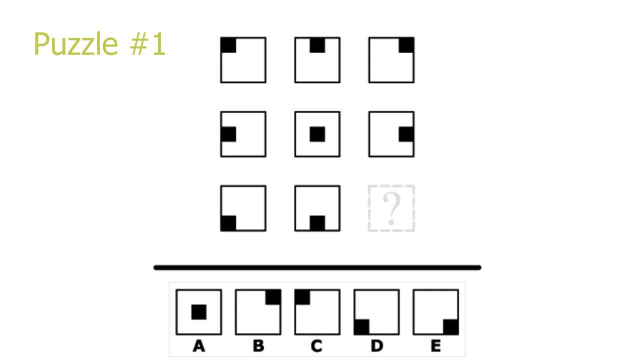 Puzzle number one: This is our one column puzzle. so if we look at the columns, we have that every picture in column one has a black square on the left side. every picture in column two has a black square on the right side. every picture in column two has a black square on the left side. 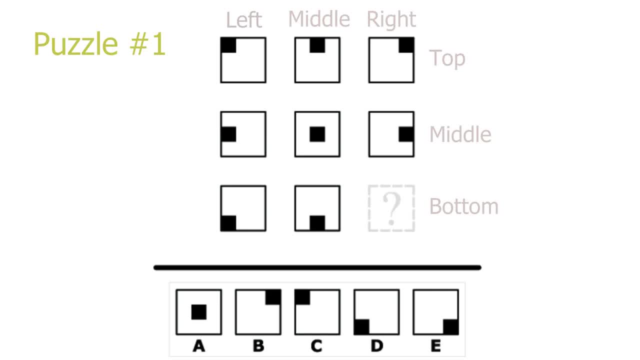 a black square in the middle and every picture in column three has a black square on the right side. For the rows we have only black squares on the top for row one, in the middle for row two and on the bottom for row three. Our answer is in the third column and third row. 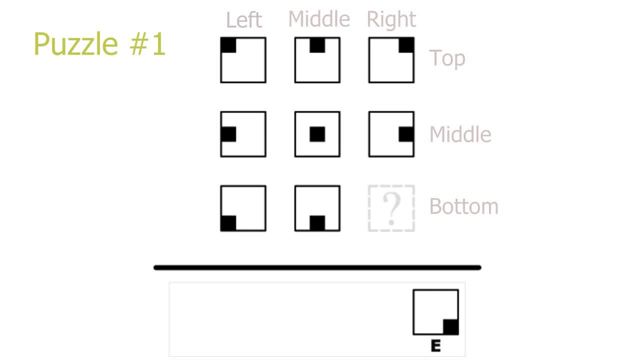 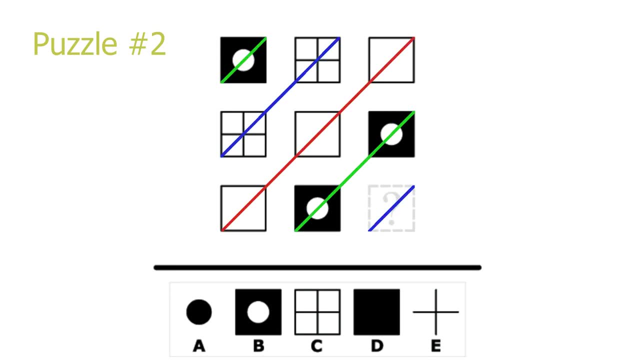 so the answer will have a black square on the bottom right. The correct solution is E. Puzzle two. This is what I call a diagonal puzzle. If we look at the diagonal from top right to bottom left, we see that every picture in a diagonal is identical. Also, we see that the diagonal 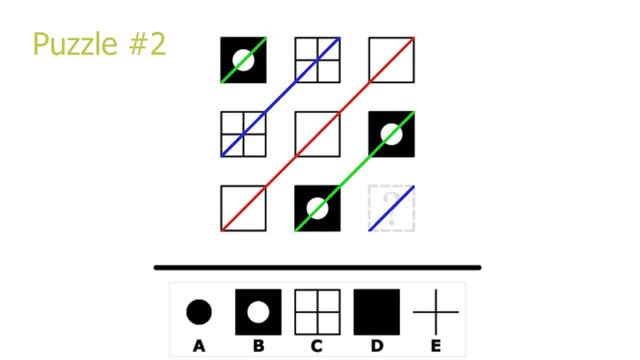 from top right to bottom left is the same as the diagonal from top left to bottom right. The first diagonal, marked in green, is identical to the fourth diagonal, which is also marked in green. Therefore, we know that the picture in the answer is identical to the pictures in the blue diagonal. 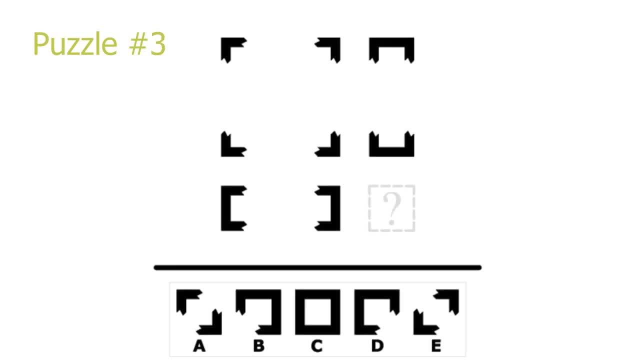 C is the correct solution. Puzzle number three: This is an addition puzzle. First let's look at the rows. So every third picture in a row can be deduced by taking the first picture in that row and adding it with the second picture. The same holds true for the columns. Every third picture in a column is the first picture. 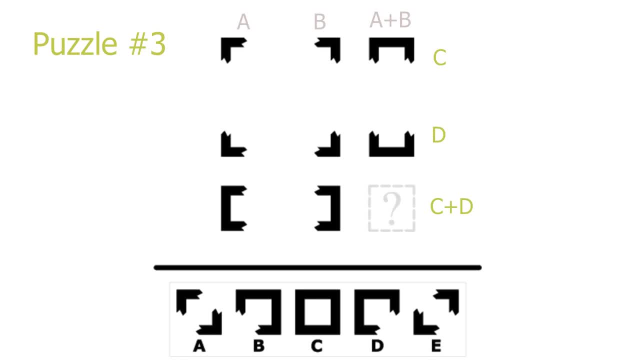 added with the second picture. So, basing ourselves on the last row, we see that if we add picture seven with picture eight, we get a fully black square. The correct answer is C. Also, we could have gone with the last column to add picture three with picture six to again get a fully black. 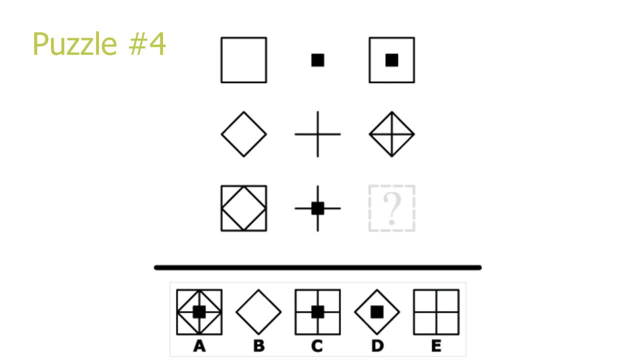 square. Puzzle number four: Another identical addition puzzle, Again in the rows. we have that picture three is picture one, added with picture two, And the same for the columns. Picture three in a column is picture one, added with picture two. Going by the last row we add picture seven with picture eight to get a square with a rotated. 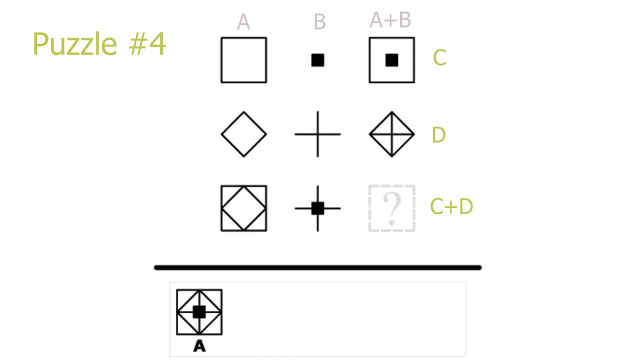 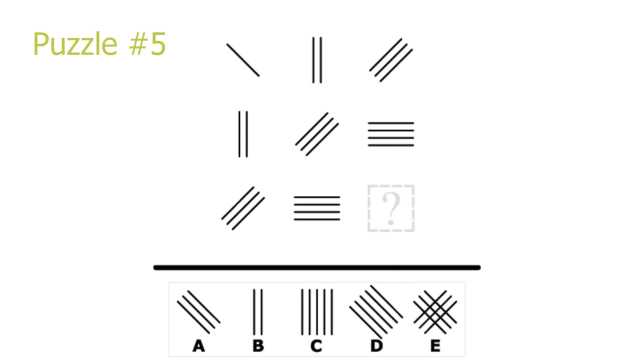 square inside of it, with a small black square in the middle and then a plus sign. So the correct solution is A Puzzle five. These kinds of puzzles have a very nice symmetry. The same change happens in the rows and the columns. To solve this puzzle, let's first take a look at the amount of lines. 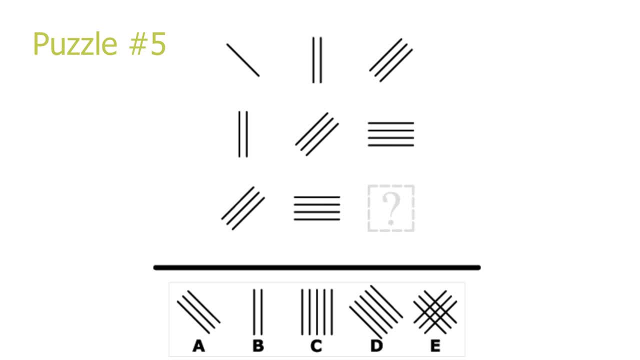 In the rows. we always add one line when we go from a previous picture to the next picture. We can write this as: plus zero for the first picture, plus one for the second picture and plus two for the third picture. The exact same thing happens in the columns, So plus zero, plus one and plus two. 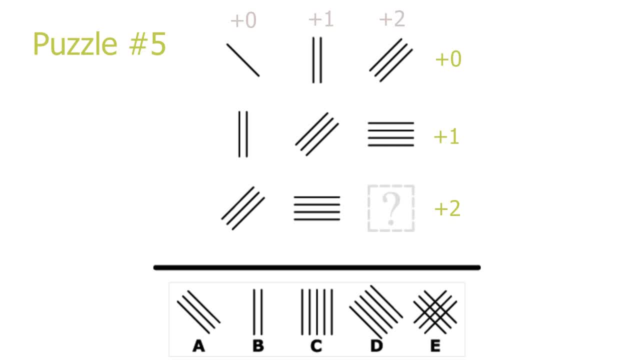 So taking the amount of lines in picture six or picture eight and then adding one line gives the amount of lines in the answer. So four plus one equals five. Our answer will have five lines. This leaves C or D as the correct answer. Also notice that, moving to the right, 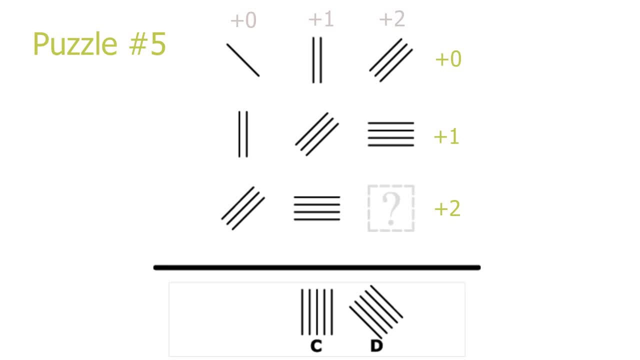 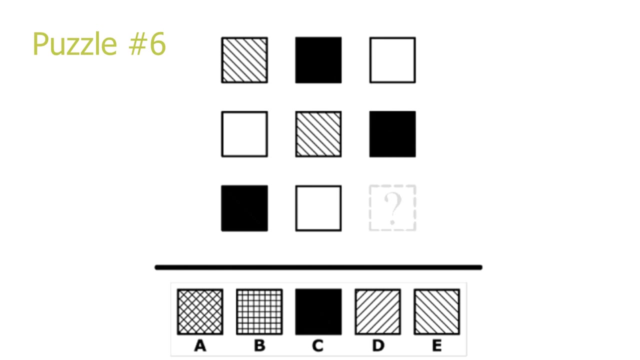 in a row or moving down in a column always leads to a 45 degree rotation clockwise. So again, take picture six or picture eight and rotate it 45 degrees clockwise to get the orientation of our answer. D is the correct solution. Puzzle six: This is a diagonal puzzle, but this time the diagonal. 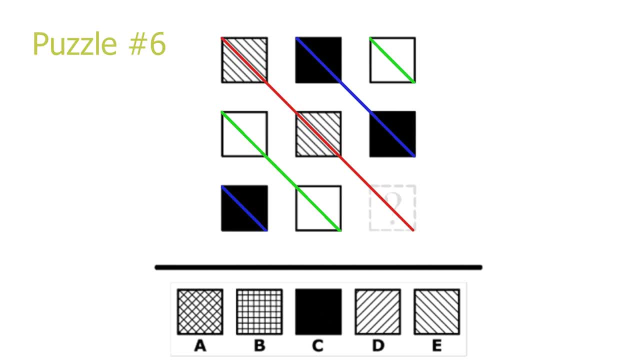 of repeating pictures is from the top left to the bottom right, Every picture in the main diagonal, which is the red diagonal, is identical. Therefore our answer is E. E is the correct solution. Puzzle seven: This is a column puzzle. So looking at the columns, we have that in column one, the black area, 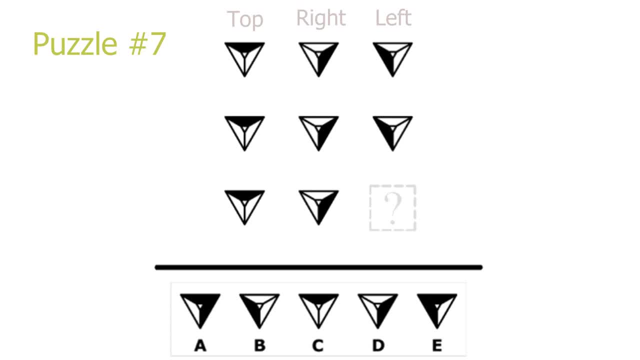 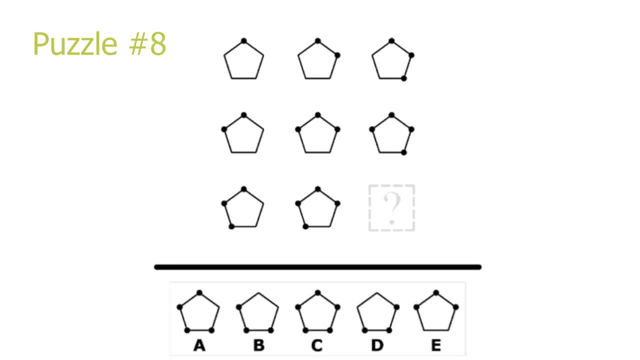 is on the right and in the third column the black area is on the left And of course every picture in a column is identical. So B is the correct solution. Puzzle number eight: Again, let's use the same logic as puzzle five. If you look at the rows, the amount of dots is always increasing by. 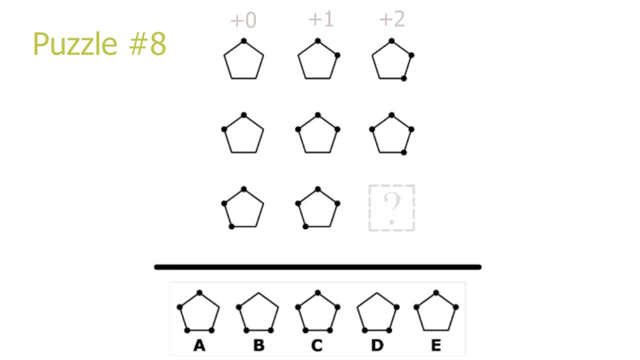 one if you move to the right, And in the columns the amount of dots always increases by one if you move downwards. So since there are four dots in picture six and picture eight, we know that the answer will have five dots. Therefore, every corner of the pentagon will have a black area. 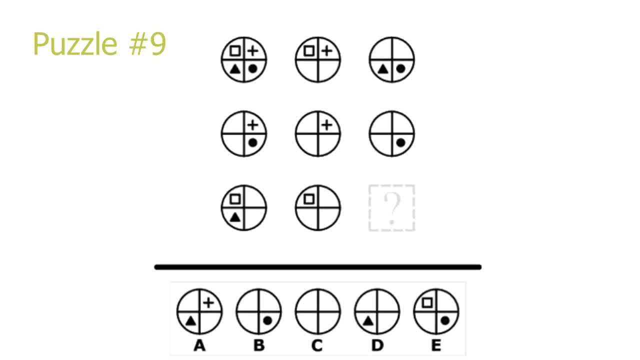 Puzzle nine. This is an addition puzzle, but here we have that in the rows, the first picture is the second picture added with the third picture. Also in the columns, the first picture is the second picture added with the third picture. So, going by the last row, we can take picture seven and remove. 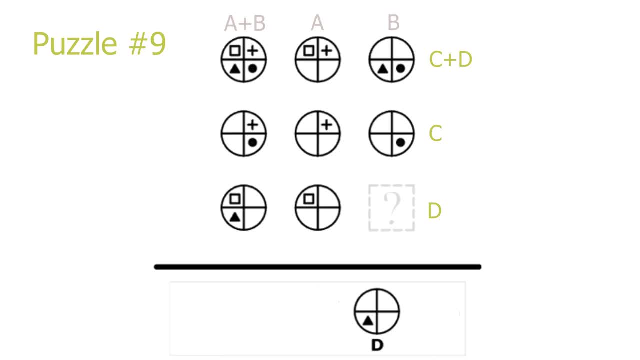 the square which is in picture eight, resulting as D as the correct solution. Also, we could have gone by the last column and take picture three and remove the circle which is in picture six and again get D as the correct solution. Puzzle nine: This is an addition puzzle, but here we have. 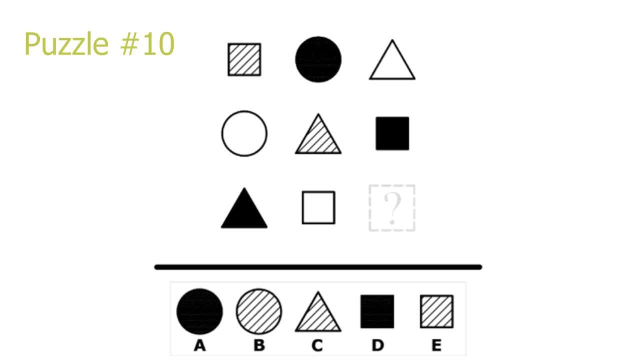 that in the rows the first picture is the second picture added with the third picture. Also, we can take picture seven and remove the square which is in picture eight and again get D as the correct solution. Puzzle ten: This is a diagonal puzzle on both diagonals. First let's look at the top left to. 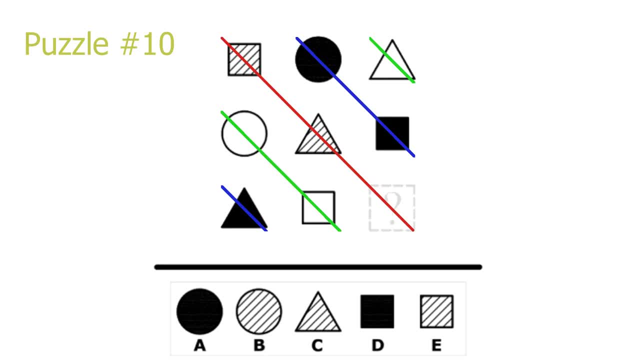 bottom right diagonal and we see that the pattern inside the shapes repeat. On our main red diagonal we have the line pattern repeating, leaving B, C or E as the correct solution. Looking at the top right to bottom left diagonal, we see that the shapes themselves repeat The repeating shape on the blue. 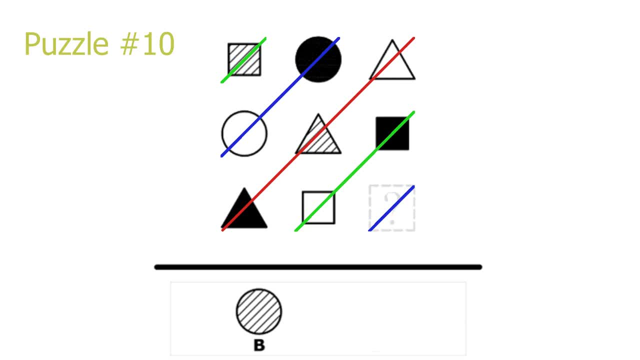 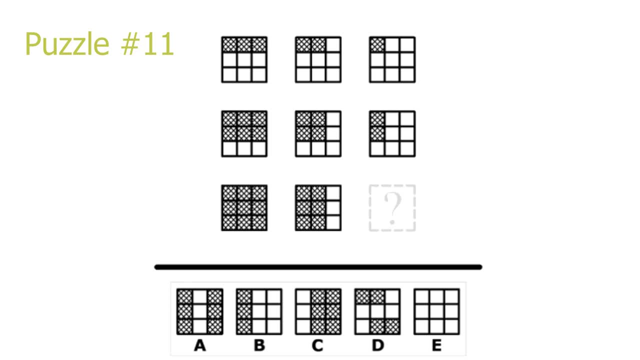 diagonals are the circles. Therefore, our answer is a circle with a line pattern inside of it. B is the solution, Puzzle 11.. This is a round column puzzle. Let's start by looking at the columns. In the first picture there is colored tiles, in all the columns. In the second column, there are 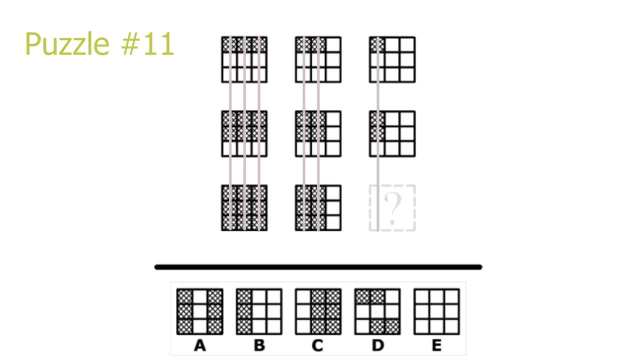 only colored tiles in the left and middle column And in the third column there are only colored tiles in the left column. If you look at the rows, In the first row there are only colored tiles in the top row. In the second row, there are only colored tiles in the top row and middle row. 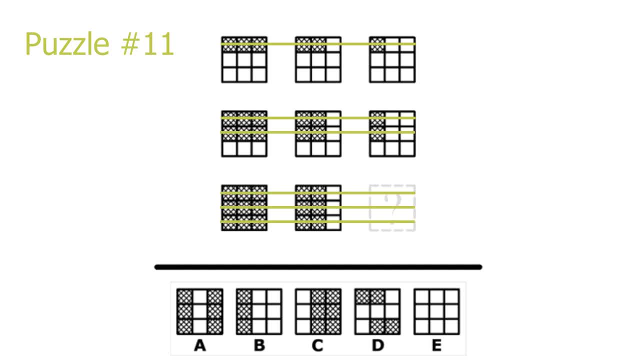 And in the third row there are colored tiles in every row. So by combining the patterns in the rows and the columns we see that there are only colored tiles where the patterns allow it. So in the lines I drew you can see that there are only colored tiles in the intersection of these lines. 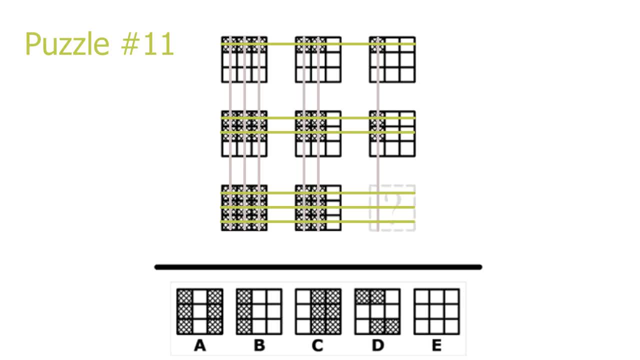 So our solution is in the third column and third row. In the third column we have only colored tiles in the left column, And in the third row we have colored tiles in all rows, Meaning that the solution will be three colored tiles in the left column. 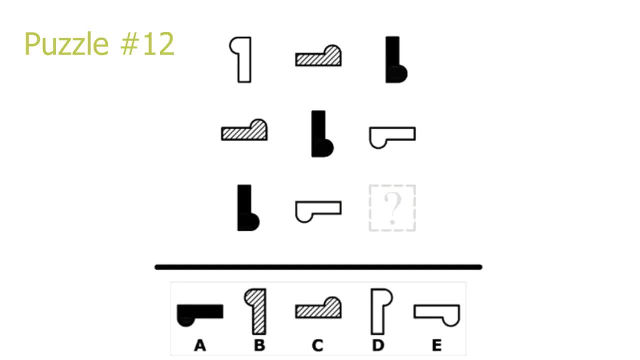 B is the graph Puzzle number 12. This is a diagonal puzzle. First, if you look at the pattern inside of the shapes, it repeats every three diagonals, leading to our answer having a line pattern. This leaves B or C as the correct solution. Note that the way the shapes are pointing does not repeat every three diagonals. So 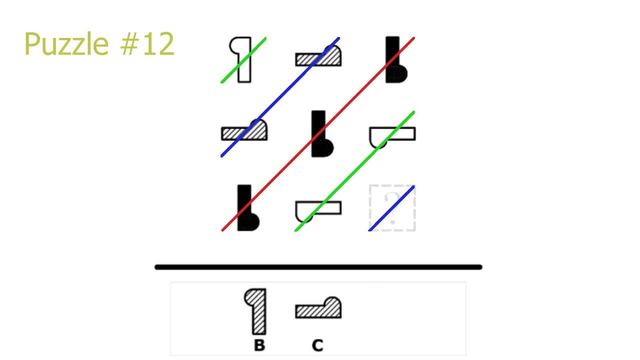 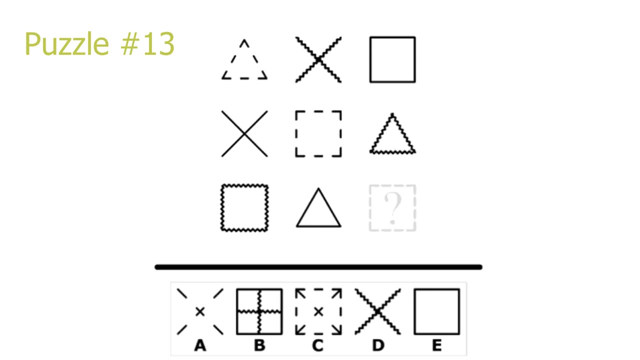 moving down a column or to the right in a row always leads to a 90 degree rotation clockwise. Basing ourselves on picture 6 or picture 8, we can rotate them 90 degrees to get the orientation. B is the correct solution. Puzzle 13.. Another diagonal puzzle, on both diagonals. First, if you look at the top right to bottom left diagonal, we have a repetition of the shapes themselves, leading to our answer being an X. 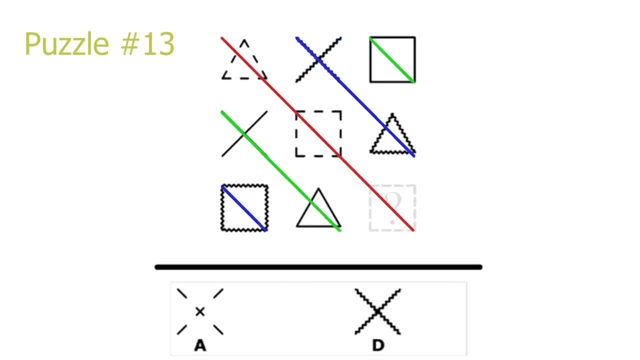 Looking at the top left to bottom right diagonal, we see that the pattern the shapes are made out of repeats. On the main red diagonal there is a repetition of the small lines which build up the shape. So our answer is: an X shape built up of small lines. A is the correct solution. 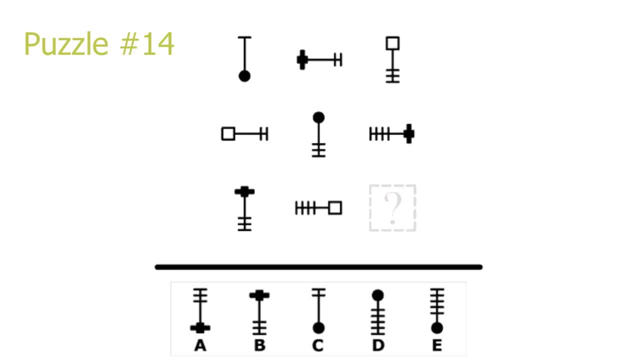 Puzzle 14.. This is a diagonal puzzle which is very similar to puzzle 12.. First let's look at the top left to bottom right diagonal and we see that there is a repetition of the object which is attached to the end of the line. In the main red diagonal there is a repetition of 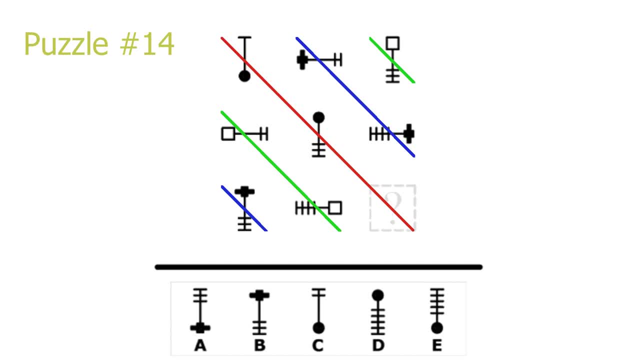 the pictures with a black circle attached to the end of the line Leading to C, D or E as the correct answer. Now, if you look at the row, we see that moving from left to right in a row always adds one of these small lines and rotates the object by 90 degrees. 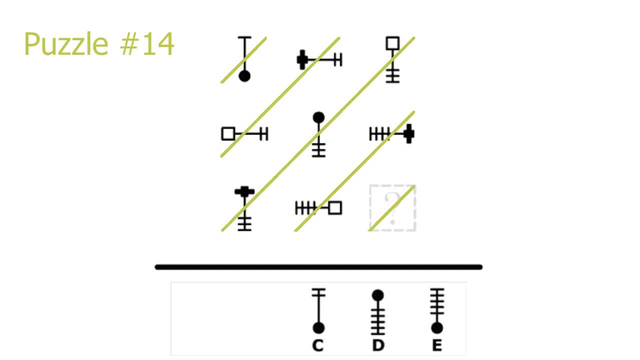 Also moving down in a column, also rotates by 90 degrees and adds a small line. So basing ourselves on picture 6 or picture 8 and rotating them 90 degrees clockwise and then adding one of these small lines leads to how this picture looks without the black circle attached to it. 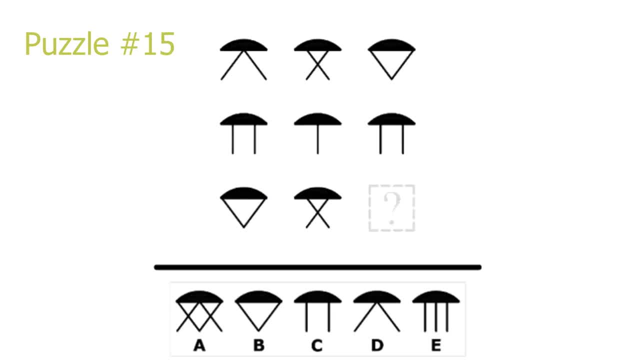 E is the correct solution. Puzzle 15.. This is a row and column puzzle. The first thing to notice is that the lines under the semicircle is always connected to one of 5 places on top and one of 5 places on bottom. 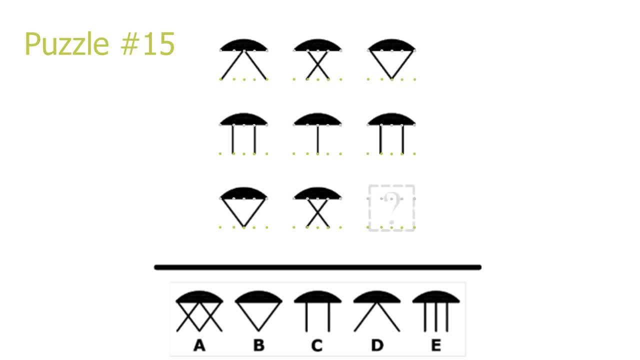 The dots I've drawn in represent these positions, these positions which the lines can be in between. To solve the puzzle, let's look at the rows and notice that there is a pattern which the left most line in the first picture always follows, And when going from a previous picture to our next picture in a row, these lines always jump. 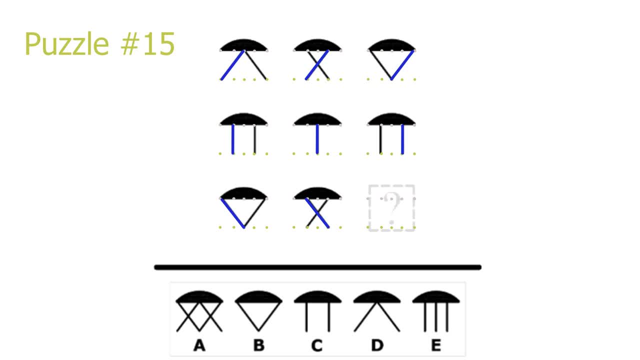 one dot to the right. So if we take the blue line in picture 8 and move it one to the right, we get one of the lines in our answer. The next thing to notice is that the right most lines which add around in red here, they always do the exact opposite of the blue line and jump one position. 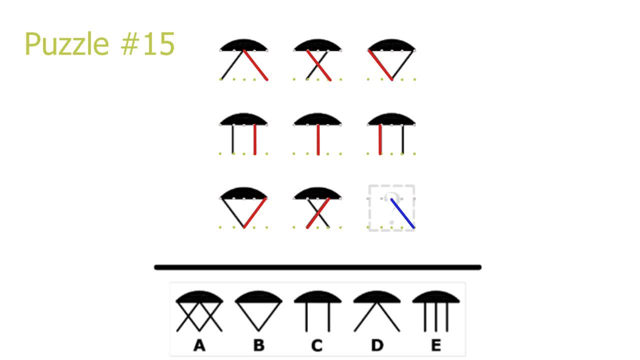 to the left as we move to the right. So if we take the red line in picture eight and move it one to the left, we get another line in our answer. So if we look at this shape, which our answer has, only d has this shape. so d is the correct solution. Puzzle 16.. Another addition puzzle. 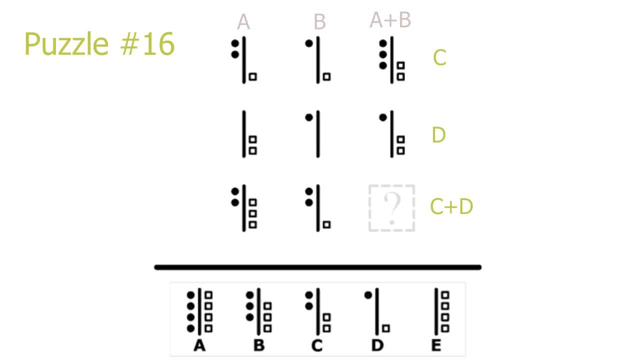 for the rows, the last picture is always the first picture added with the second picture, And for the columns, the last picture is always first picture added with the second picture. This becomes quite obvious if you look only at the black dots In the first row. we have one black dot in the first picture and two black dots in the 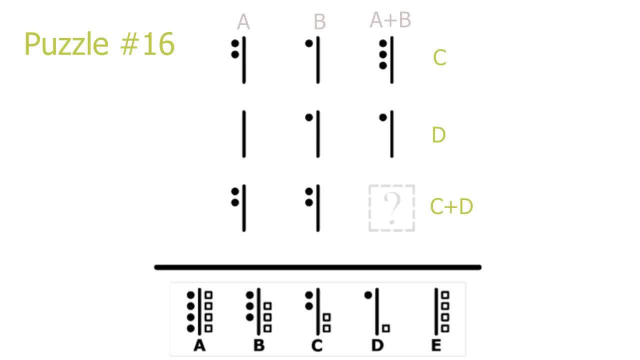 second picture, and this adding of black dots works for every column and every row. The same holds true for squares. For the last row, we have two plus two black dots, so four black dots, and three plus one squares, so four squares. A is the correct solution. Puzzle number 17.. This is another puzzle. 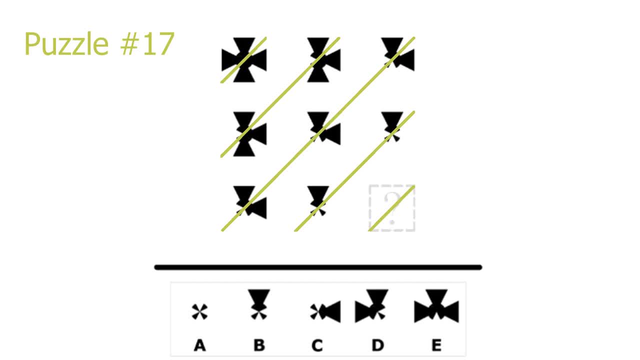 where moving to the right in a row or moving down on a column has the same effect. This effect is that it always removes one triangle from our answer. So, basing ourselves on picture 6 or picture 8, we see that they only have one of these triangles left. so if you remove it, we get the. 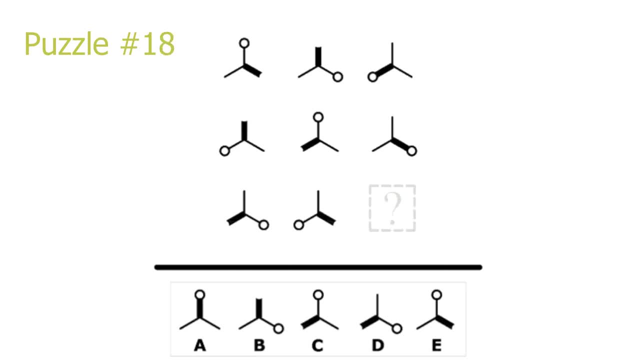 correct solution. So A is the correct solution. Puzzle number 18.. This is a diagonal puzzle on both diagonals. First, if you look at the top left to bottom right diagonal, we see that there is a repetition of where the circle is attached onto the shape. For the right triangle we see that the 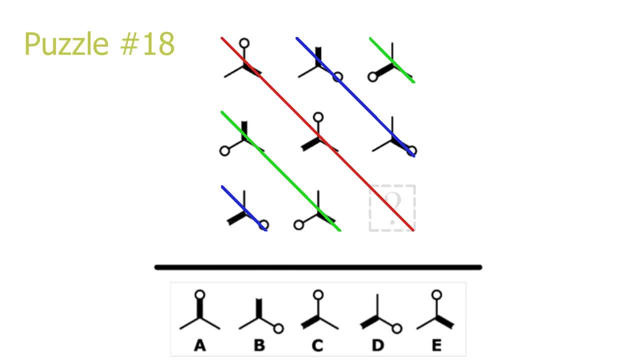 main red diagonal, the circle is always attached to the top. This leaves A, C or E as the correct solution. If you look at the top right to bottom left diagonal, there is a repetition of where the thick black line is For the blue diagonal, which corresponds to our answer. we see that the thick 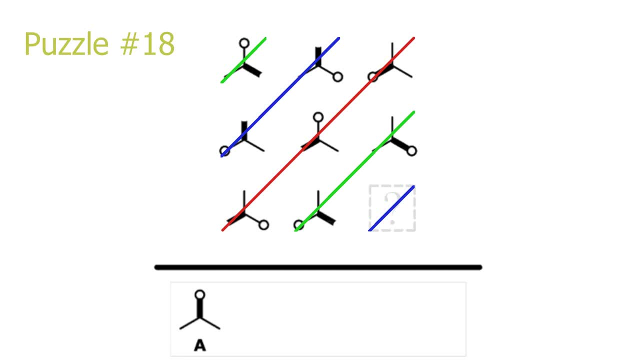 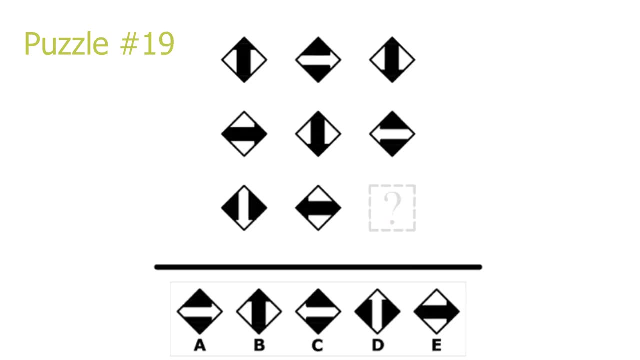 black line repeats on the top. So our answer has a thick black line on the top with a circle attached to it. A is the correct solution. Puzzle number 19.. This is a diagonal puzzle. First let's look at the top. left to bottom, right diagonal. This is a diagonal puzzle. First let's look at the top, left to bottom. 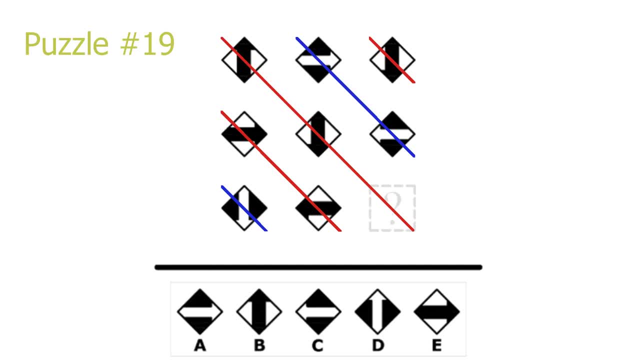 right diagonal, On the diagonals which I've drawn as red, there are only pictures which are white with black arrows, and in the blue diagonals there are only black pictures with white arrows. The answer is in the main red diagonal, so it will be white with a black arrow, meaning that B or E is the 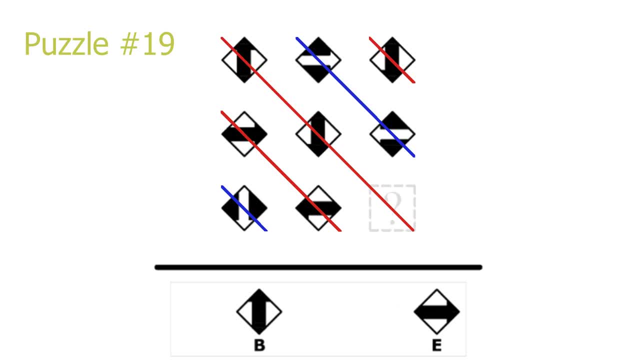 correct answer. Again, there is a 90 degree clockwise rotation when you move to the right in a row or downwards in a column. So basing ourselves on picture 6 and picture 8 and rotating it 90 degree clockwise, we get the orientation of our answer. 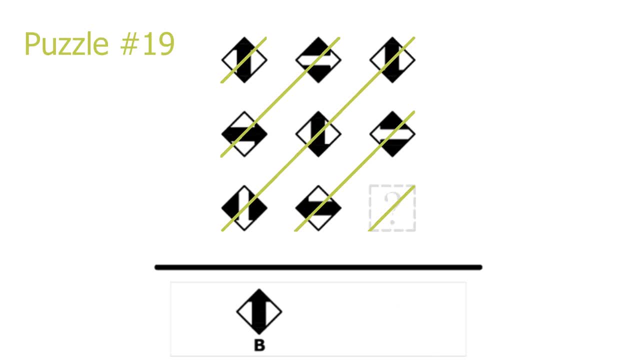 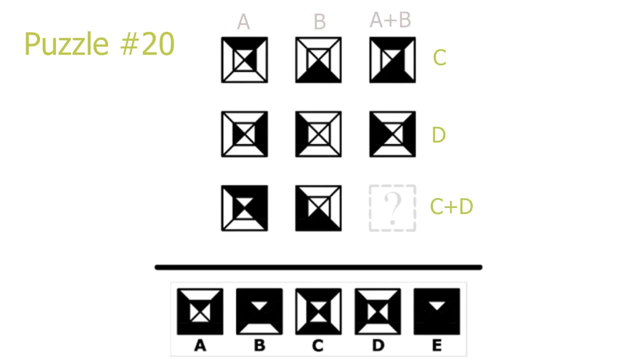 So the answer is an arrow pointing upwards. B is the correct solution. Puzzle 20.. This is a simple addition puzzle of the black areas. On the rows, the last picture is the first picture added with the second picture, And on the columns, the third picture is the first picture added with the second. 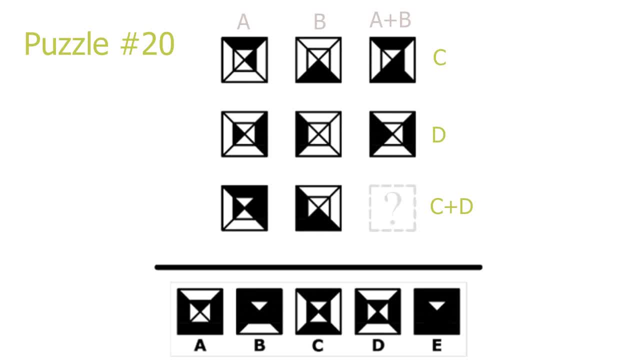 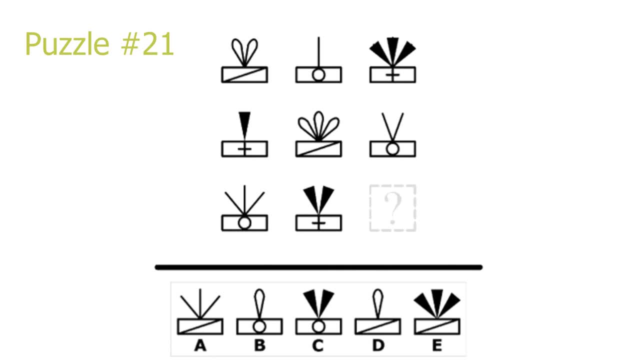 picture. So, basing ourselves on the last row or column, we see that adding the black areas together gives us E as the correct solution. Puzzle 21. This is a diagonal puzzle on both diagonals. First let's look at the top right towards the bottom left diagonal. 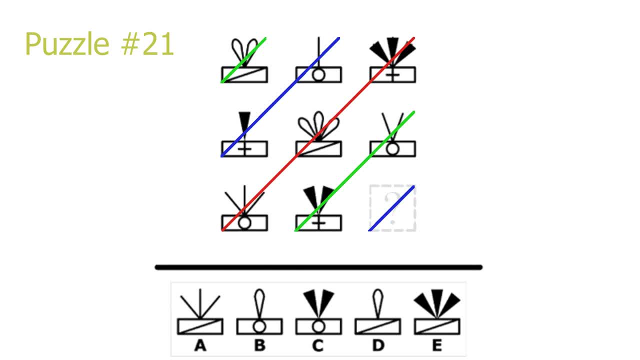 We see that how many objects stick out of the top of the picture repeats? On the blue diagonal, which our answer is in, there is a repetition of one object sticking out of the top. This leaves B or D as the correct solution. If we look at the top left to bottom right diagonal, we see a repetition of 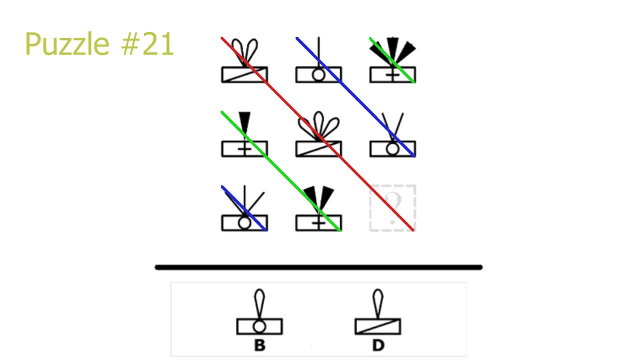 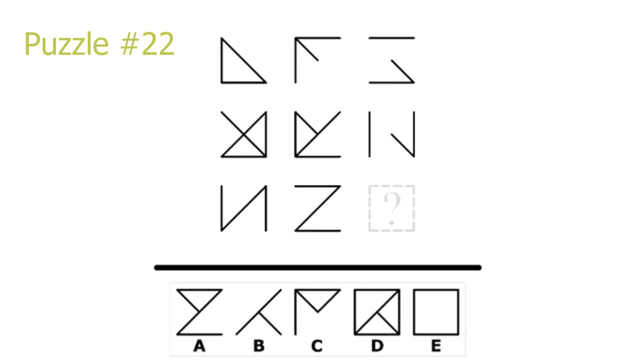 what object sticks out of the top and what shape is inside of the rectangle? The pattern inside the rectangle on the red diagonal is a line from the top right corner to the bottom left corner. This D is the correct solution. Puzzle 22.. This is an addition puzzle with cancellation. 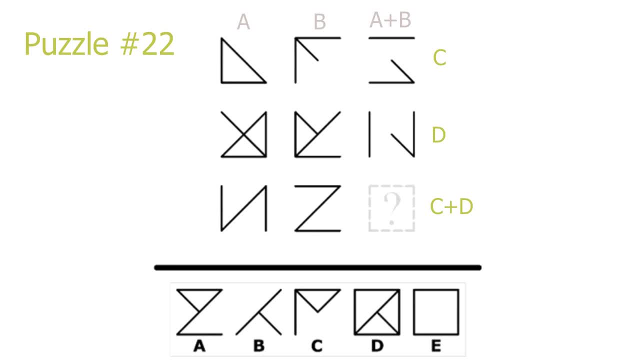 So it's regular addition where the last picture is the first picture added with the second picture both in the columns and the rows. But what picture 1 and picture 2 has in common is removed from picture 3.. For example, if we look at the first row, we have picture 1. we place picture 2 on top of it. 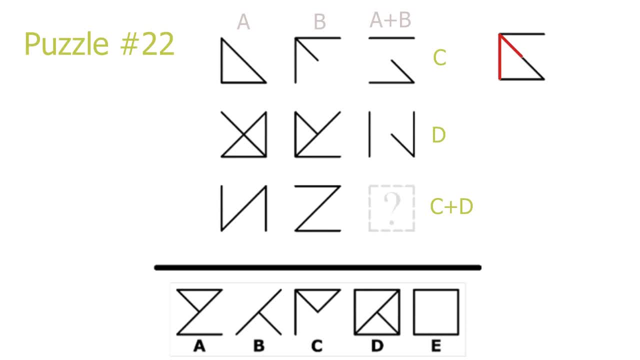 Here we can see that the red is what picture 1 and picture 2 has in common, and if we remove this, we just do the same process for the last row. We add picture 7,, we add picture 8, we have this overlaps which is marked in red, and we remove the red to get our answer. E is the correct solution.